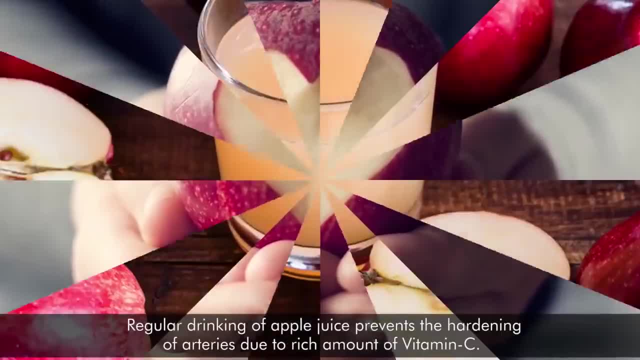 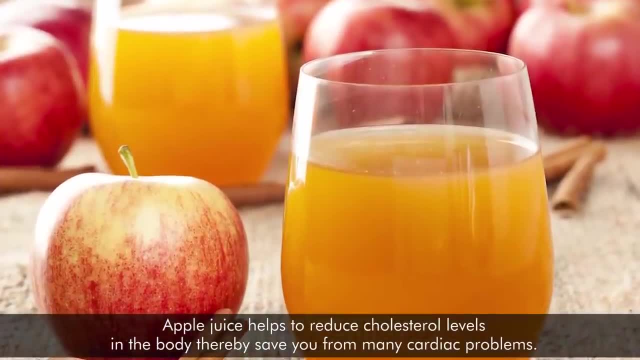 Regular drinking of apple juice prevents the hardening of arteries. due to rich amount of vitamin C, Apple juice helps to reduce cholesterol levels in the body, thereby save you from many cardiac problems. 3. It prevents joint pain. Apple juice is good for the heart. 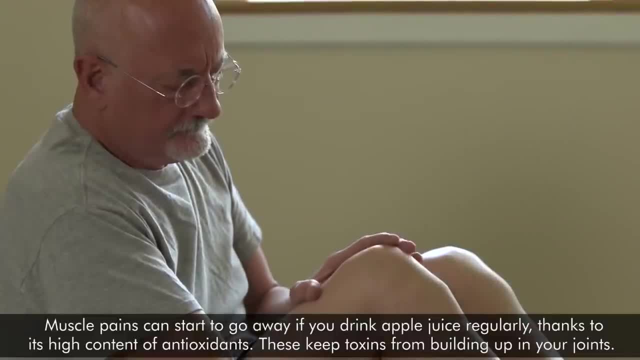 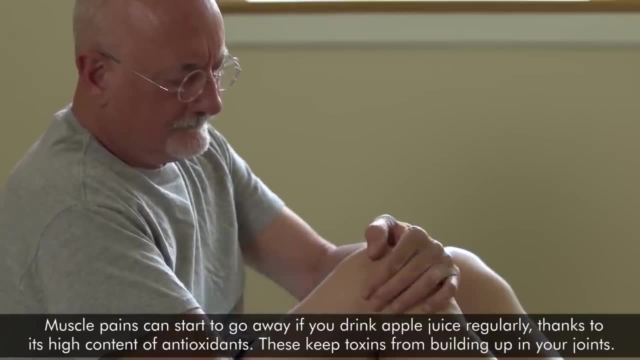 Apple juice is organic, producing vitamins that improve sexual conditioning ó It prevents joint pain. Muscle pains can start to go away if you drink apple juice regularly. thanks to its high content of antioxidants, These keep toxins from building up in your joints. Thanks to this, you can start drinking it to stop spoiling your health as well. 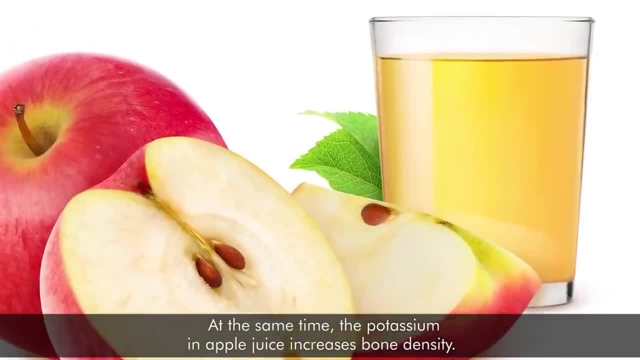 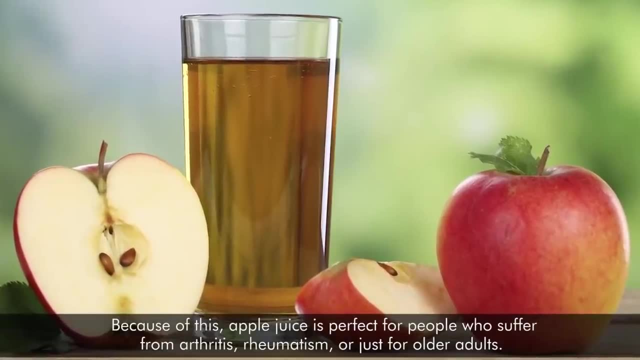 At the same time, the potassium in Apple juice increases bone density. Because of this, apple juice is perfect for people who start suffering from arthritis, rheumatism, or just for older adults. 4. Apple juice for liver health. Apple juice is a healthyелей, albeit highVones, drug-free. brain-eugia-остоqing is bestαςauer'. Apple juice somatology hypoglycemia can help liver health. Apple juice provides vitamin C. Apple juice is very good for blood circulation and bowels. Apple juice- egg jaw fluid type 1Small". 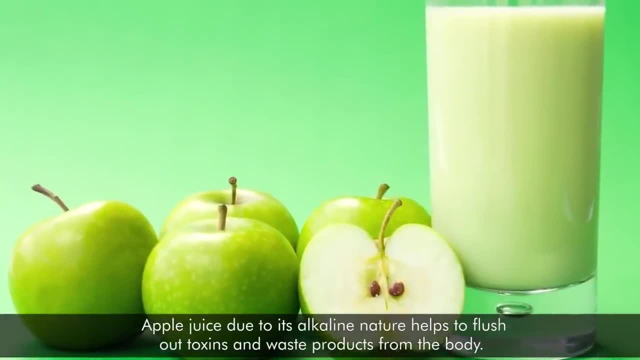 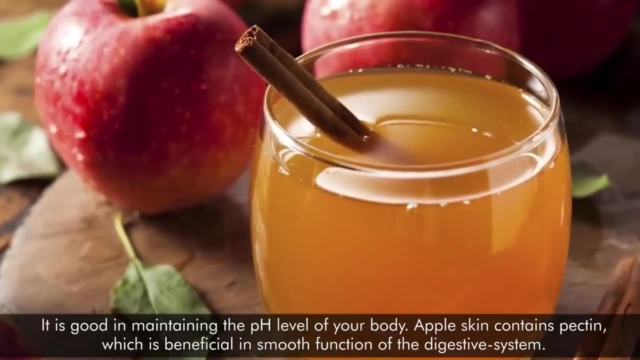 alkaline nature helps flush out toxins and waste products from the body. It is good in maintaining the pH level of your body. Apple skin contains pectin, which is beneficial in smooth function of the digestive system. Thus apple juice acts like a liver cleanser. 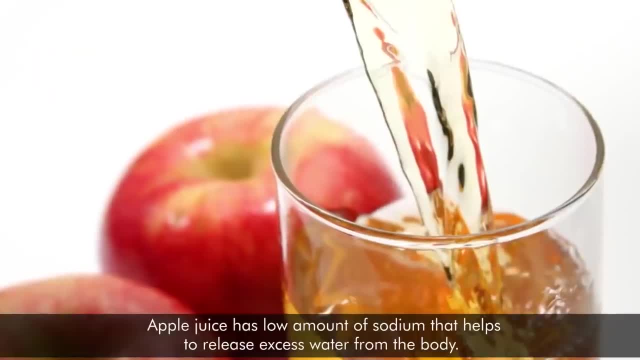 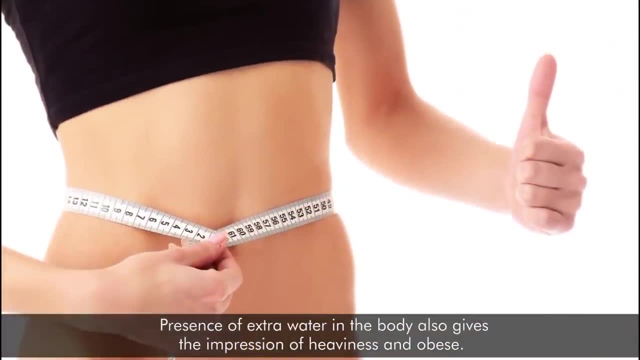 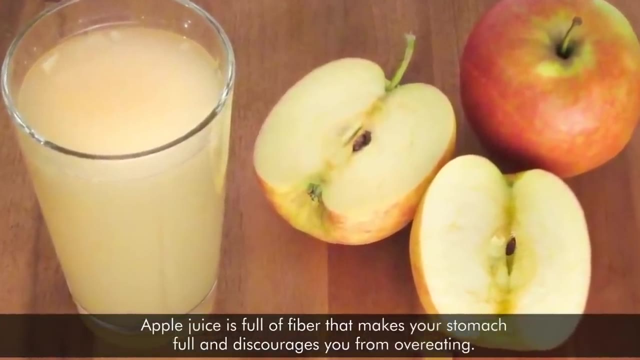 5. Apple Juice for Weight Loss. Apple juice has low amount of sodium that helps to release excess water from the body. Loss of extra water in the body also gives the impression of heaviness and obese. Apple juice is full of fiber that makes your stomach full and discourages you from overeating. 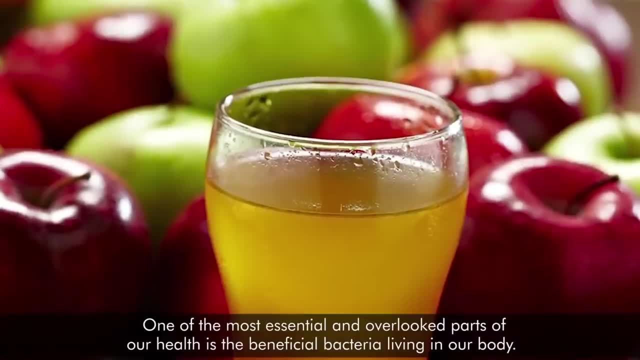 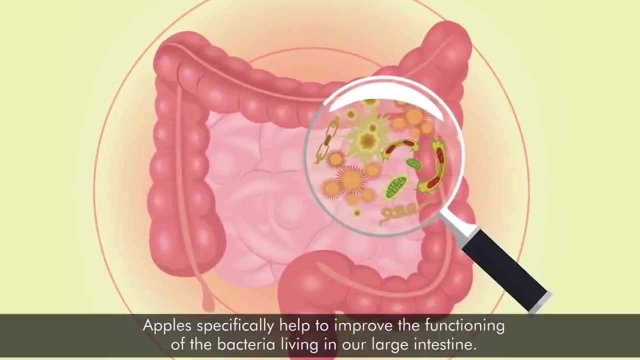 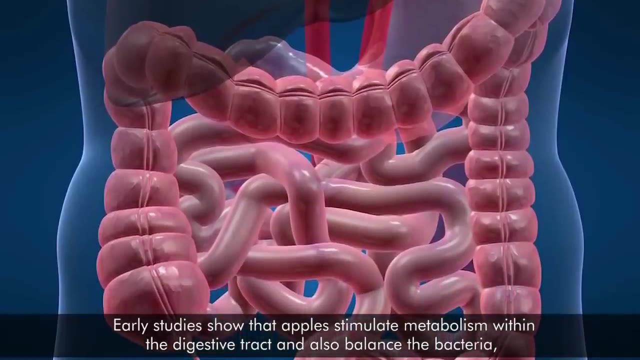 6. Improve Intestinal Health. One of the most essential and overlooked parts of our health is the beneficial bacteria living in our body. Apple specifically help to improve the functioning of the bacteria living in our large intestine. Early studies show that apples stimulate metabolism within the digestive tract. 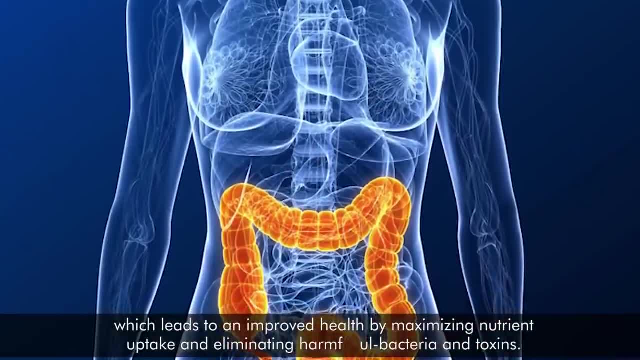 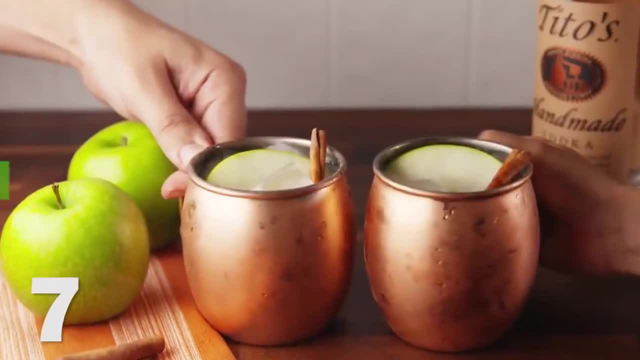 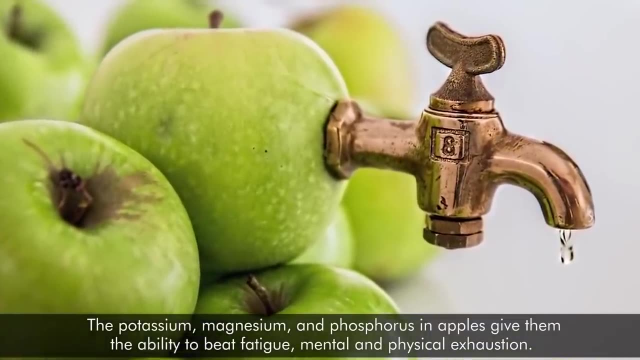 And also balance the bacteria, which leads to an improved health by maximizing nutrient uptake and eliminating harmful bacteria and toxins. 7. It Revitalizes Your Mind. The potassium, magnesium and phosphorus in apples gives them the ability to beat fatigue, mental and physical exhaustion. 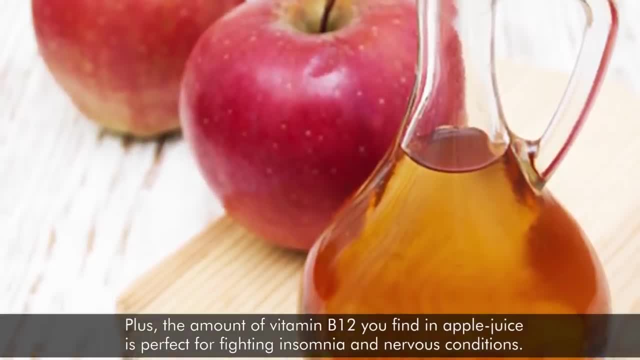 Plus, the amount of vitamin B12 you find in apple juice is perfect for fighting insomnia and nervous conditions. 7.